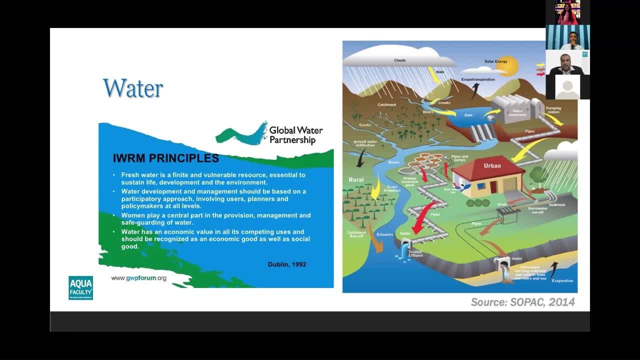 is the reason why we need to use it wisely and why we are talking about this management, because everyone knows that is a kind of finite resource. So we have the technology for converting the sea water into drinking water, but it's not so easy and price is not. 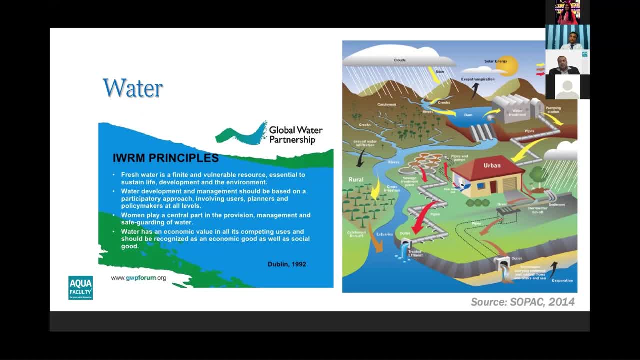 so affordable when we compare with the other water sources. So that's why water management is very important. The composition of the categories in the water cycle can be varied, but as a whole, I mean when you see this water cycle, the picture right side- I mean we know this water. 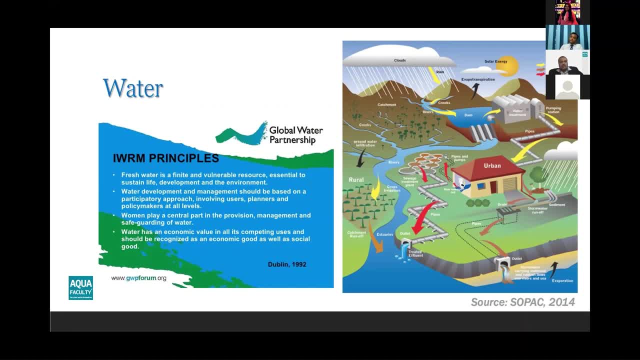 cycle from the childhood We are learning about that. We learn from the beginning. okay, the precipitation and the surface runoff and the river storming, and after that we extract water for the areas and after that we have a certain amount of wastewater. So the water. 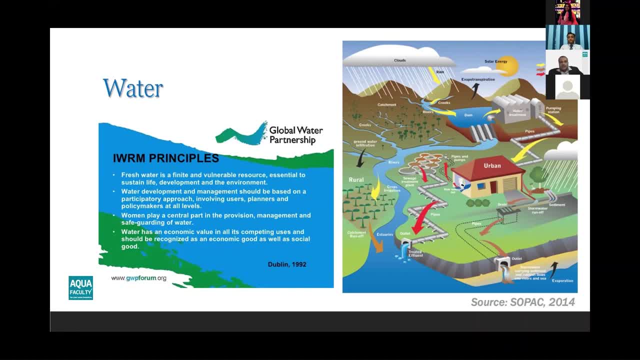 cycle goes on in different categories. The amount inside within the cycle allocated for various categories will be varied, but as a whole it's a kind of finite amount. This is why in the Dublin water summit in 1992, it was agreed to have a common water management principles. It is called integrated. 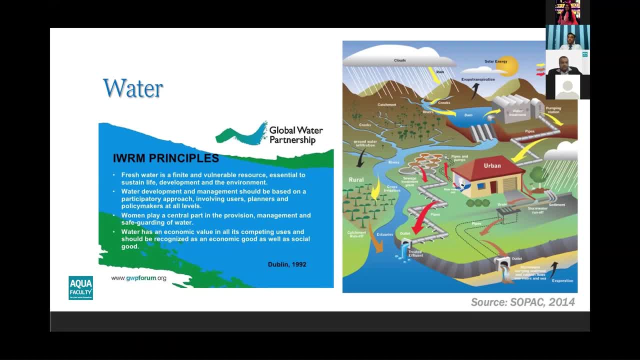 water resource management principles or Dublin principles. So we need to know about this because it's very important if you are going forward. I would like to brief it very briefly. She says the wastewater is a finite and vulnerable source, so it understand. okay, it is a finite. I mean, we know the amount. 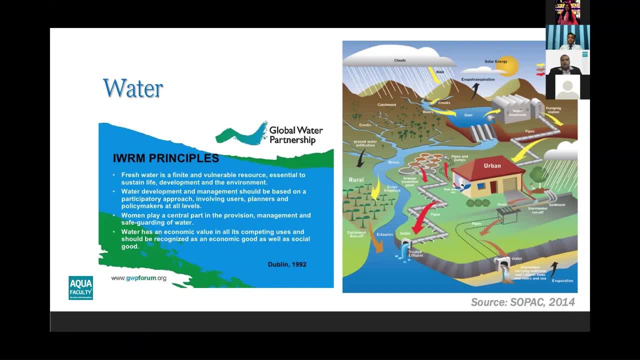 we have is finite amount. Well, that is why we need to manage it. And the second: the water development and management should be based on participatory approach, involving users, planners and politicians. bravely, However, it is necessary to scramble, Марк. 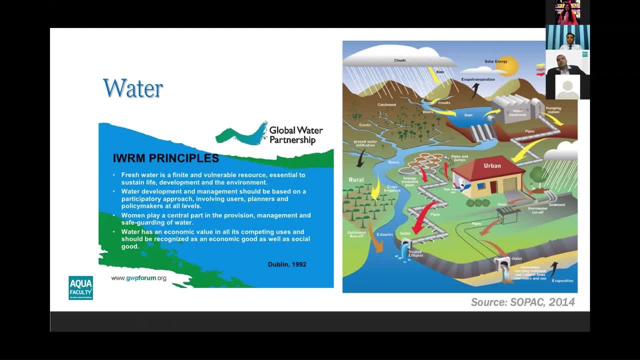 funds to manage it. That is what the domain of mixed water is like for now. So free water policymakers at all levels. so this is talking about a trick. I mean the in the integration of the participatory approach. the integration now, when we are talking about water, when we are taking